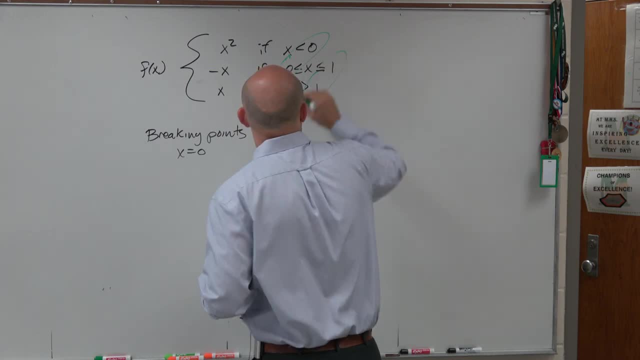 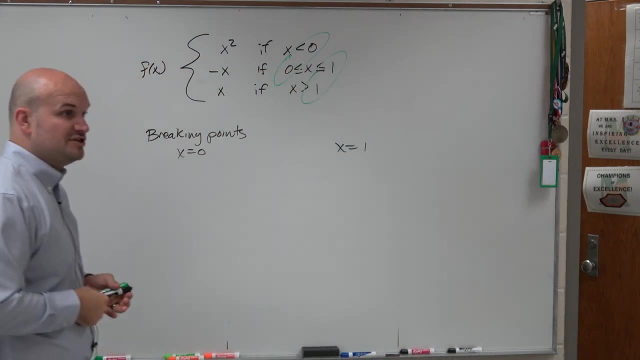 Other way to look at it. those two values, That's where these graphs, that's where they can be disjoint. So what we want to do, then, is to make sure, if this continues, we want to look at what is the limit, then, from the left. 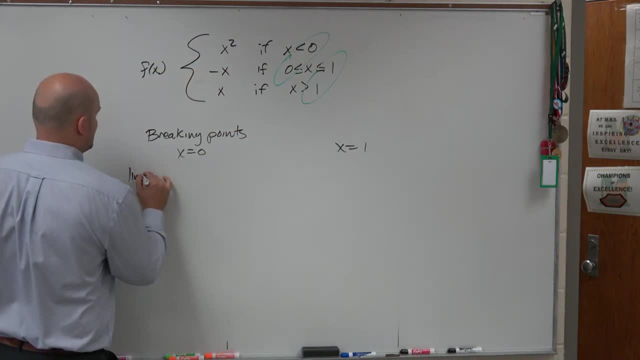 and from the right of each of those points. So we want to make sure that the limit as x approaches 0 from the left of f of x has to be equal to the limit as x approaches 0 from the right of f of x. 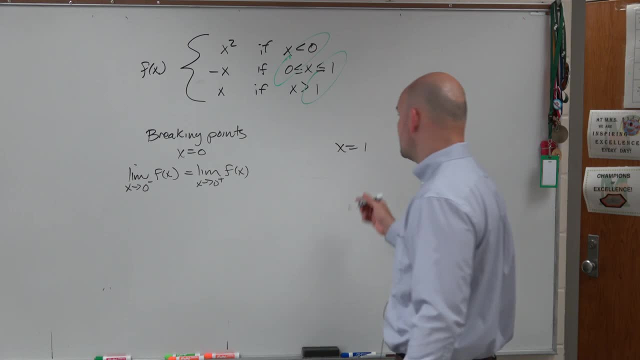 If the limits are the same, then we know that it's obviously continuous at that point. And then over here, the limit as x approaches 0 from the 1 from the left of f of x has to be equal to the limit as x approaches 1 from the right of f of x. 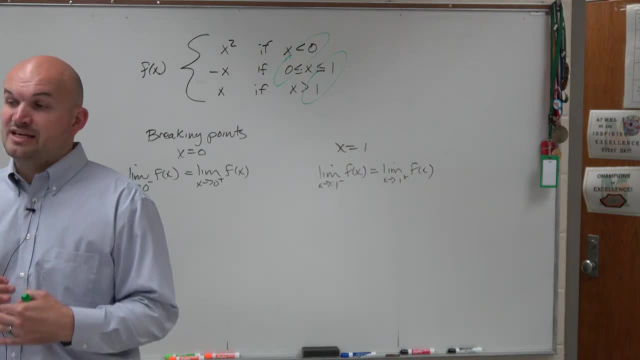 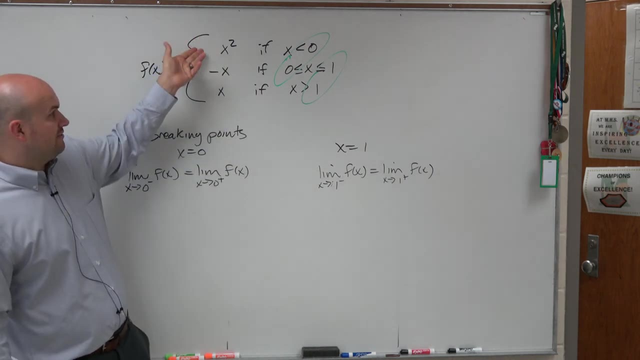 And the reason why I said: as long as the limit exists, as long as they're equal. we know the limit exists because, ladies and gentlemen, it's continuous. Let's look at these functions. Is there any reason to believe there's any discontinuities? 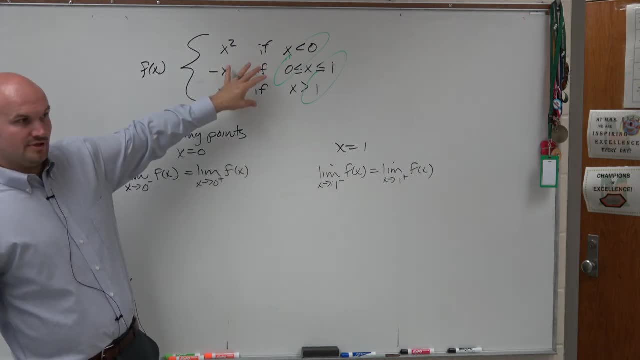 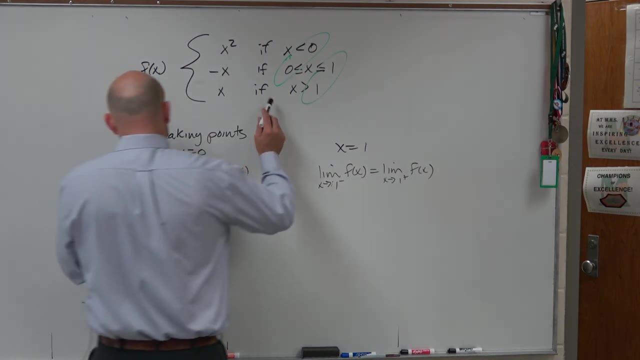 in these functions. No right, We're looking pretty good there, So we're perfectly fine with that. All we want to do now is just basically check in the left-hand limit. So the left-hand limit of 0 is going to be x squared. 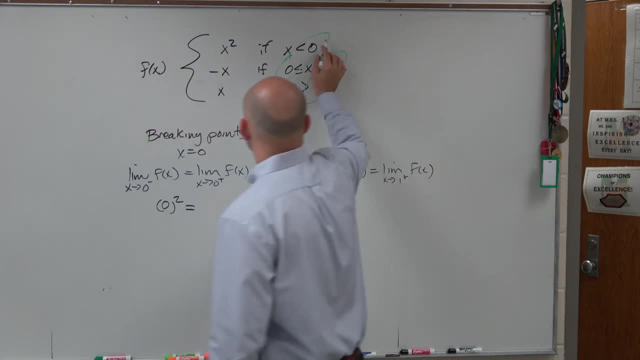 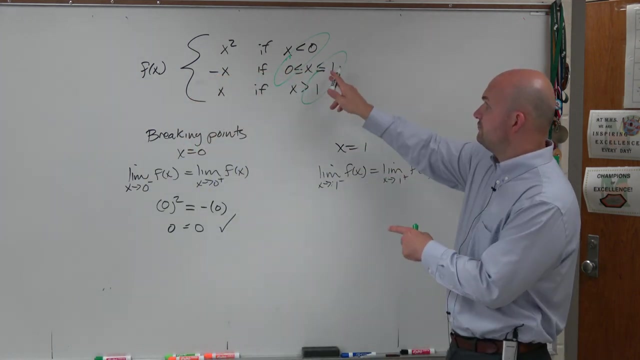 So we're going to have 0 squared has to equal the right-hand limit, which is going to be values that are greater than 0, which is negative x. Good, Then the right-hand limit or the left-hand limit of 1,. 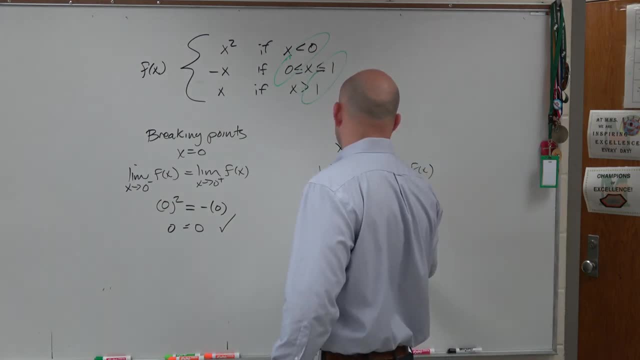 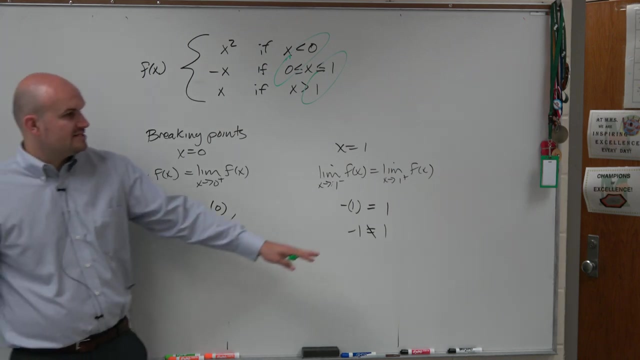 is going to be this function, which is negative 1.. So negative 1 has to equal the right-hand limit, which is just going to be 1.. So it's continuous here, but it's not continuous there. And then again, how do we know what type of discontinuity? 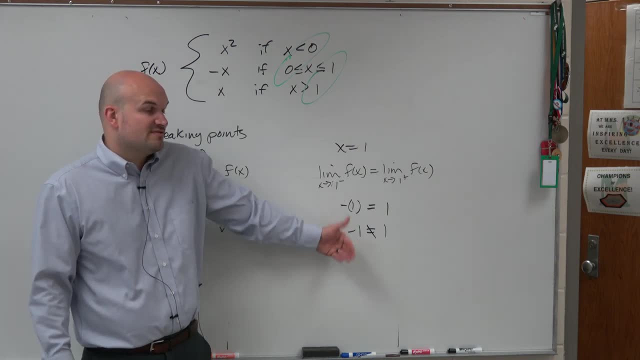 it is. We know that this is a discontinuous function because it has a jump discontinuity. One of them is at negative 1.. One of them is at 1, like we did.